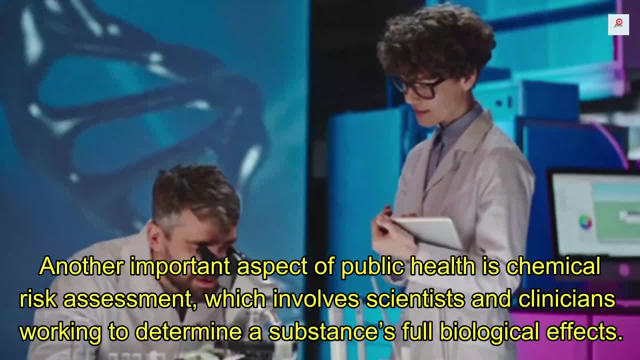 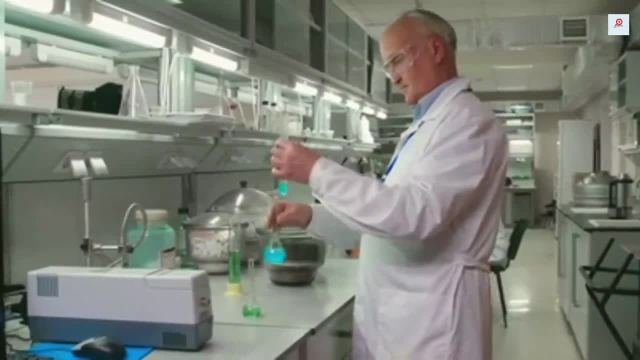 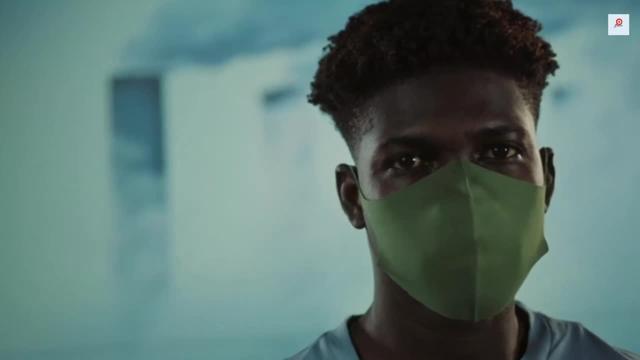 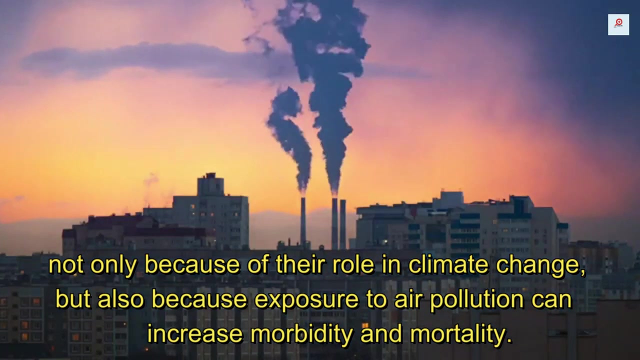 are ahem They fry together. in an email form, дости Ofong V3 darüber. effects number two: air pollution. studies have shown that air pollution effects on humans are a significant public health concern, not only because of their role in climate change, but also because of exposure to air pollution can increase morbidity and mortality when 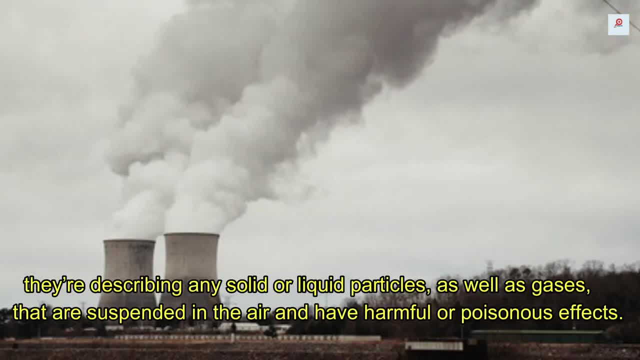 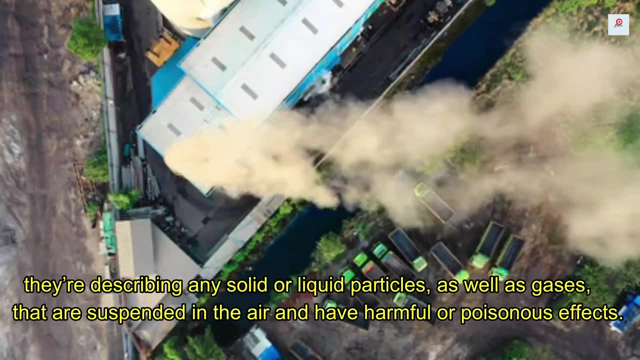 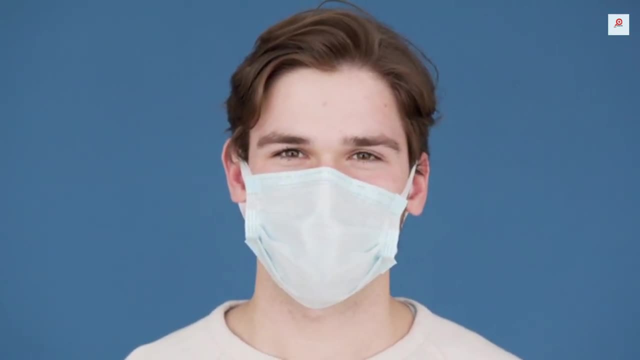 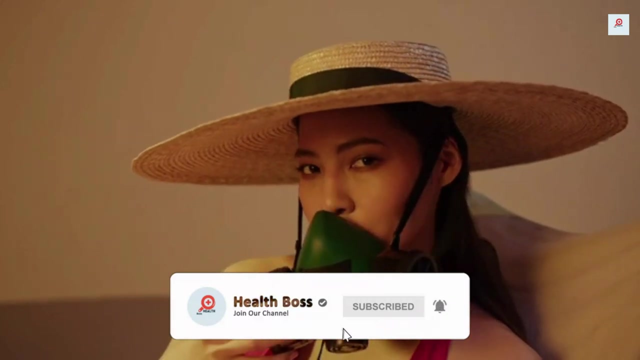 environmental scientists talk about air pollution, they are describing any solid or liquid particles, as well as gases that are suspended in the air and have a harmful or poisonous effects. when we think about air pollution, we tend to think in terms of human caused pollutants, and rightly so. some of the most dangerous and ubiquitous examples of air pollution include: 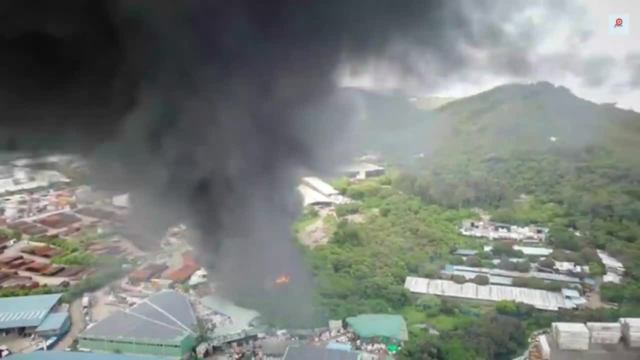 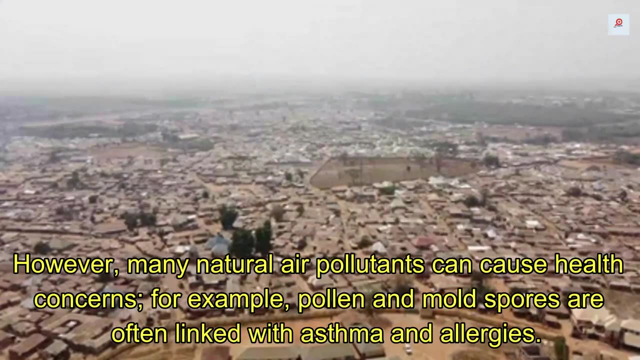 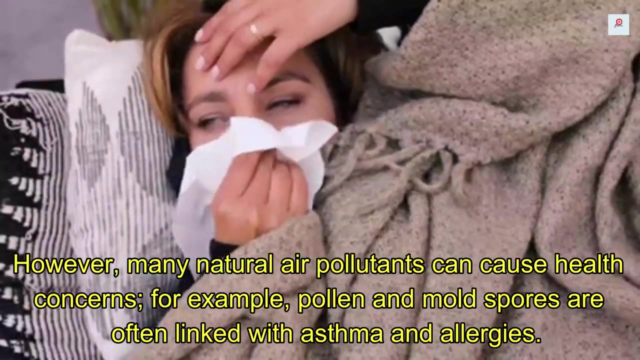 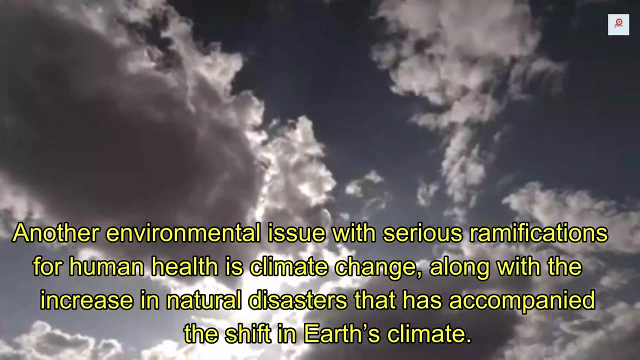 car and truck exhaust, as well as polluting byproducts of industrial processes. however, many natural air pollutants can cause air pollution health concerns. for example, pollen and mold spores are often linked with asthma and allergies. number three: climate change and natural disasters, another environmental issue with serious ramification. 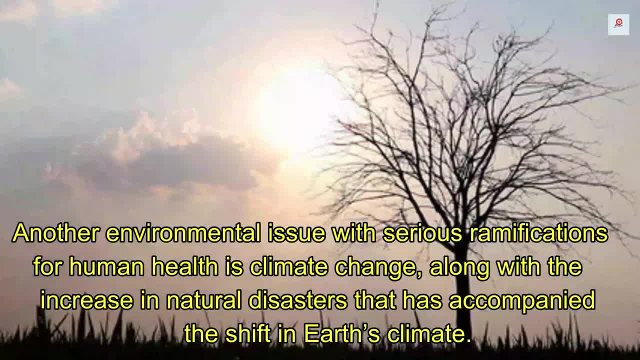 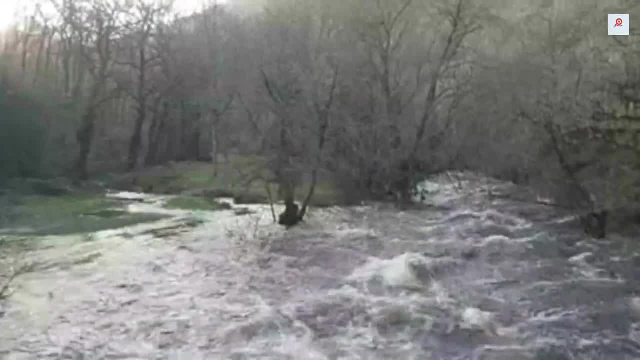 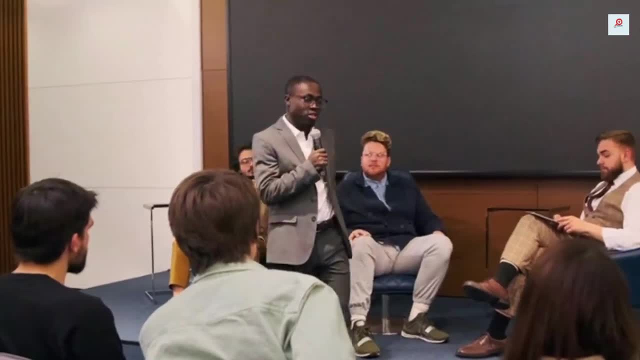 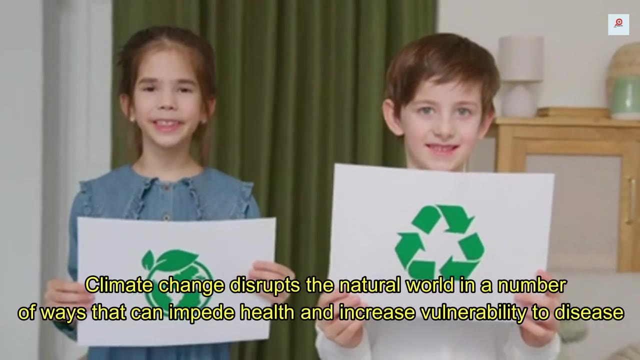 for human health is climate change. along with the increase in natural disasters that has accompanied the shift in earth's climate, the national environmental health health association lists climate change as the single biggest human health threat of the 21st century. climate change disrupts the natural world in a number of ways that can impede health. 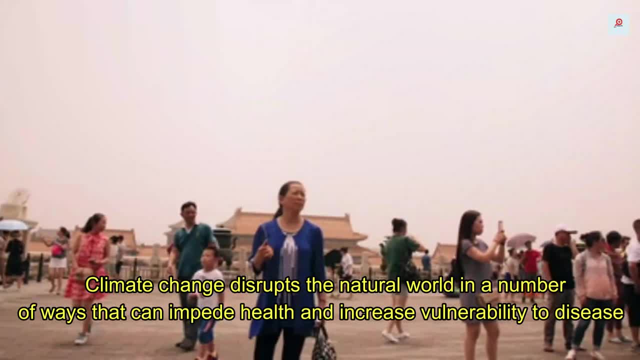 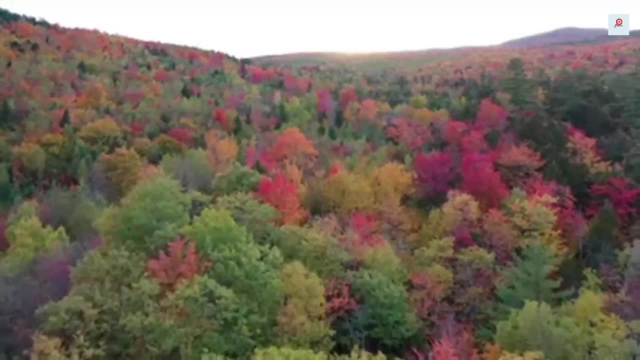 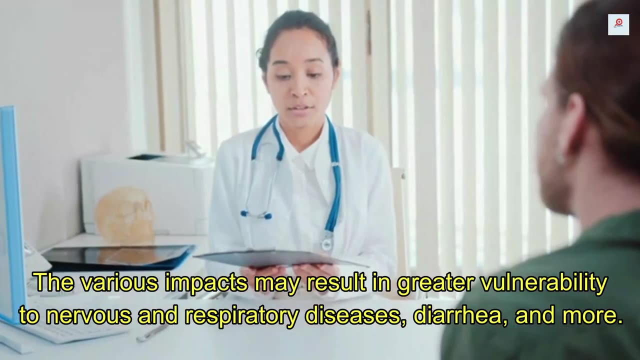 and increase vulnerability to disease. this includes increases in the planet's temperature and more frequent heavy rains and runoff. the various impacts may result in greater vulnerability to diseases such as air pollution and air pollution, as well as air pollution in the world, nervous and respiratory diseases, diarrhea and more number four diseases caused by microbes. 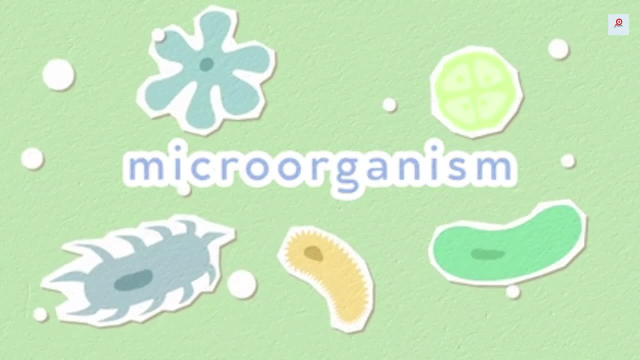 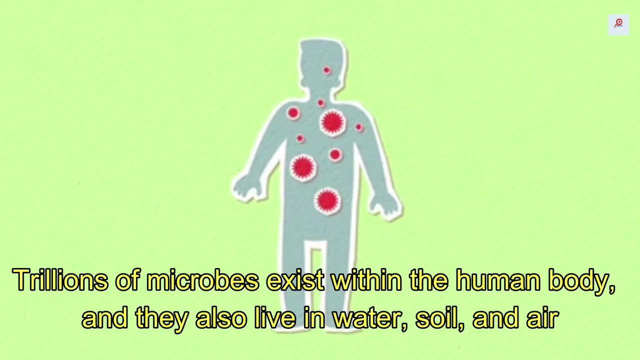 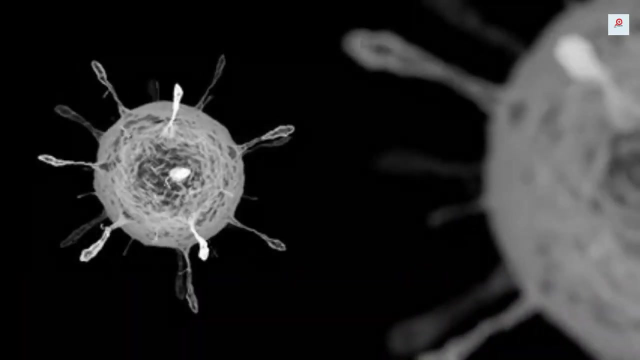 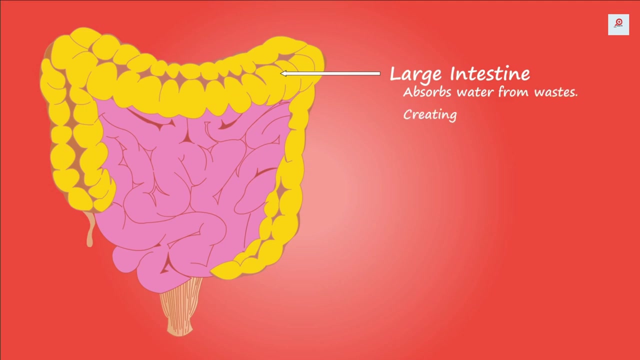 diseases caused by microbes, also known as microorganisms, present another area of public health concern. trillions of microbes exist within the human body, and they also live in water, soil and air. most of them have no negative health effects, and many microbes perform important biological functions, such as supporting digestive and immune system. according, 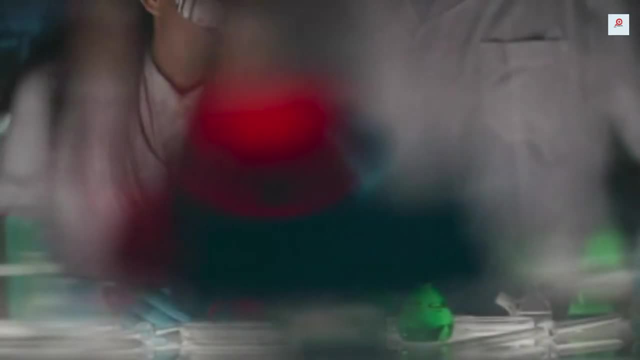 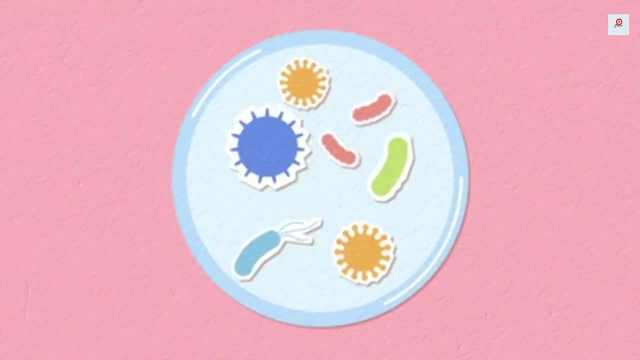 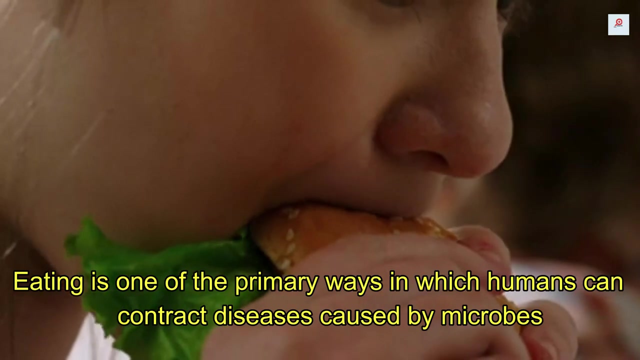 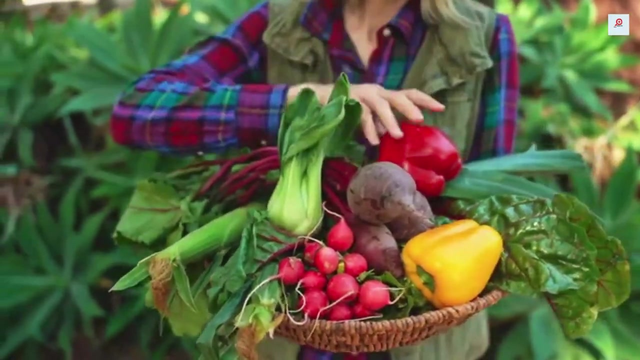 to the national human genome research institute. bacteria, viruses and fungi are types of microbes. harmful microbes, which are more commonly called pathogens or germs, can infect humans and cause illness. eating is one of the primary ways in which humans can contract diseases caused by microbes. one example is food poisoning from equally that type of bacteria that can be found in the 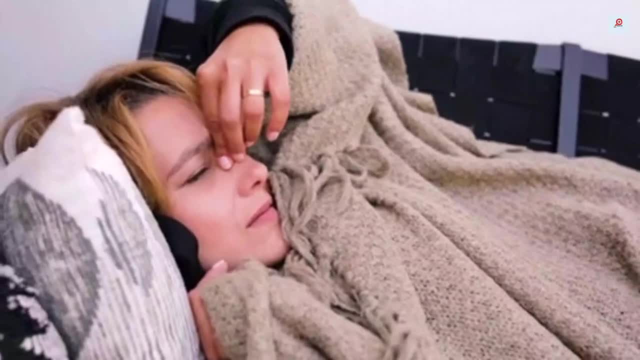 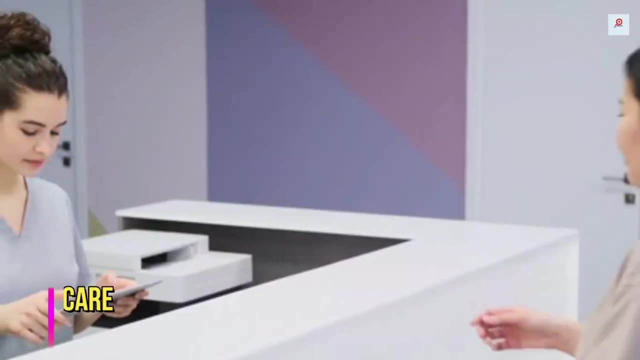 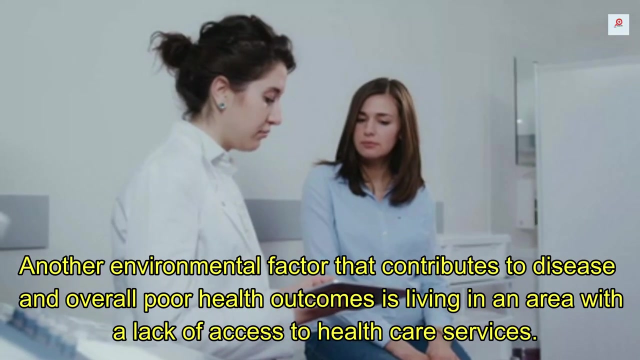 environment and in foods, and which can cause respiratory illness, urinary tract infections and other adverse health effects. number 5: lack of access to health care. another environmental factor that contributes to disease and overall poor health outcomes is living in low quality and poor health outcomes is living in low quality. health outcomes is living in low quality. 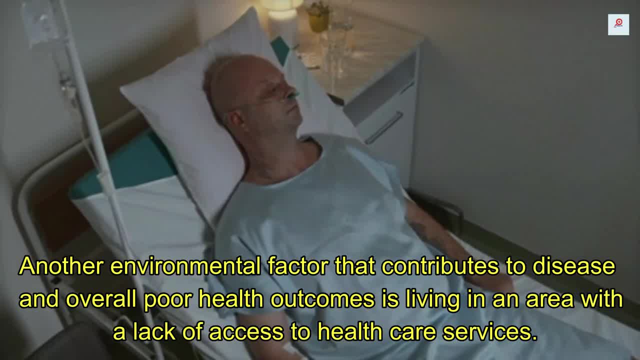 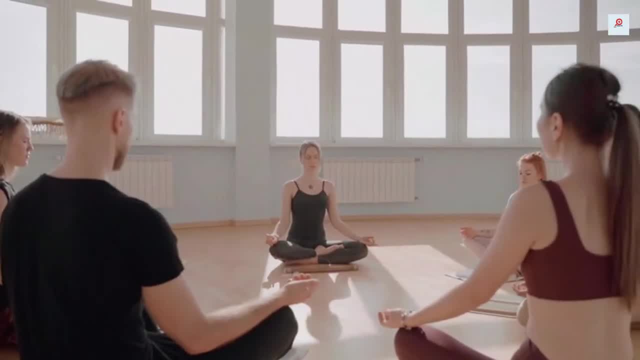 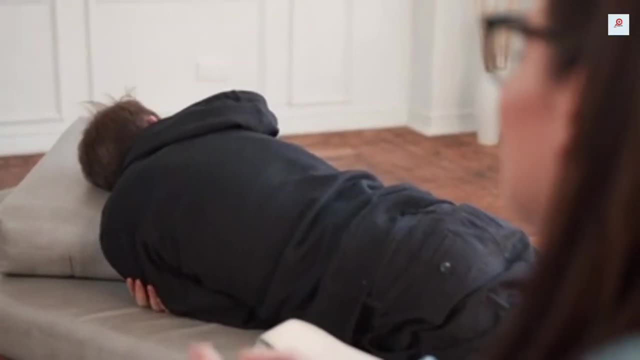 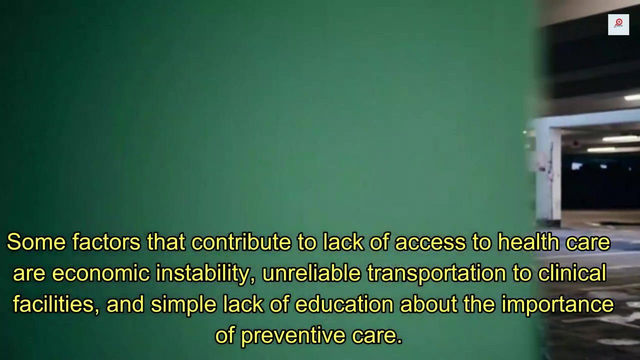 an area with a lack of access to health care services. According to the Healthy People, many people face barriers that prevent or limit access to needed health care services, which may increase the risk of poor health outcomes and health disparities. Some factors that contribute to lack of access to health care are economical instability. 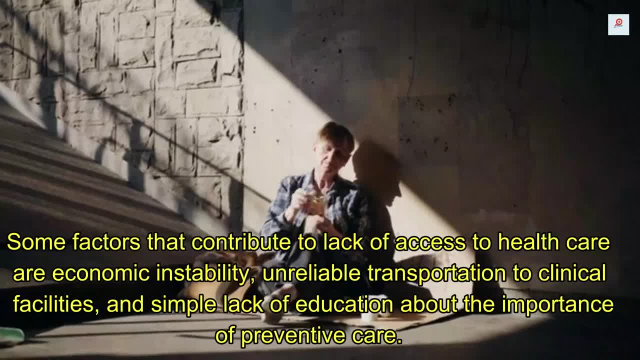 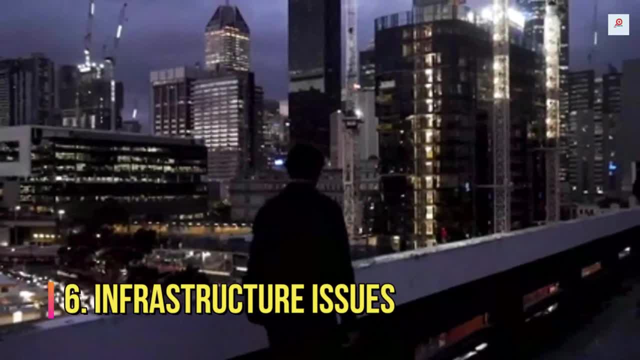 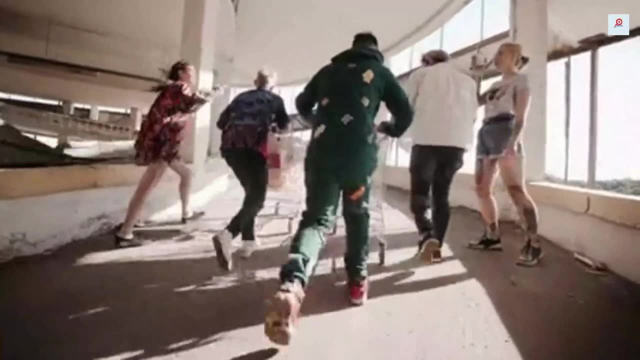 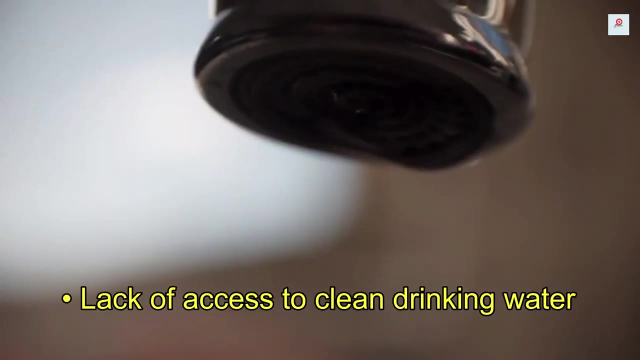 unreliable transportation to clinical facilities and simple lack of education about the importance of preventive care. Number 6. Infrastructure Issues. Infrastructure issues can also have a major impact on community health. Examples include the following: Poorly maintained roads, lack of access to clean drinking water, lack of local health.